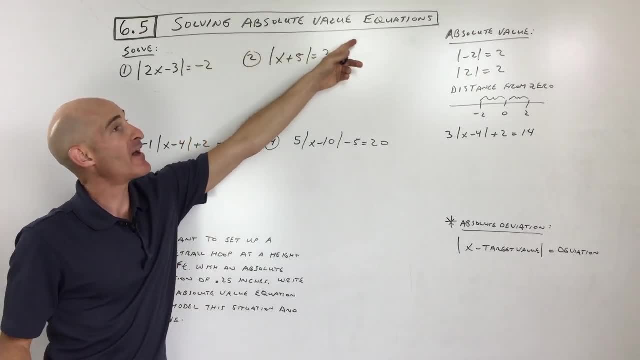 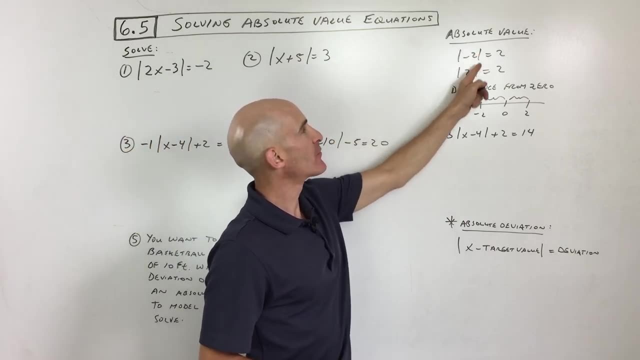 Okay, section 6.5, we're going to talk about solving absolute value equations. So remember, we talked about absolute value a while back. okay, But remember, when you see these vertical bars, that means absolute value And what it tells you is: what's the distance from zero? 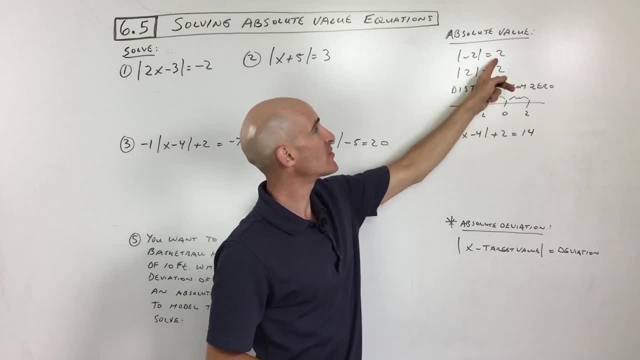 So if you look at negative two on the number line, what's that distance from zero? You can see it's two units. When you look at the absolute value of positive two, what's that distance from zero? It's two units. So when we take the absolute value, it always gives. 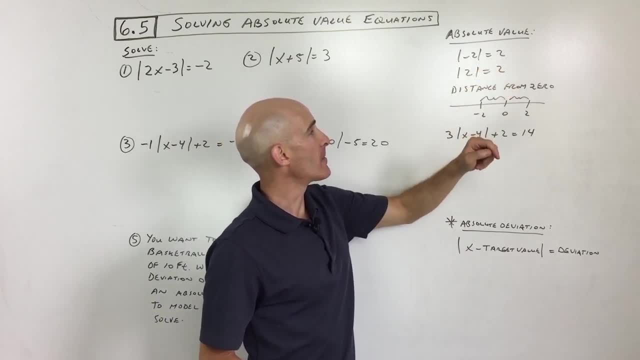 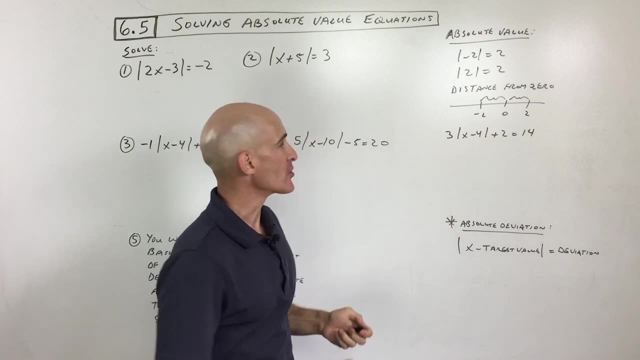 us a positive result over here. But what we're really looking at is what is the distance from zero? So let's look at an example here and I'll show you how it works. So the first thing is to isolate or get that absolute value quantity by itself. So what I'm going to do, 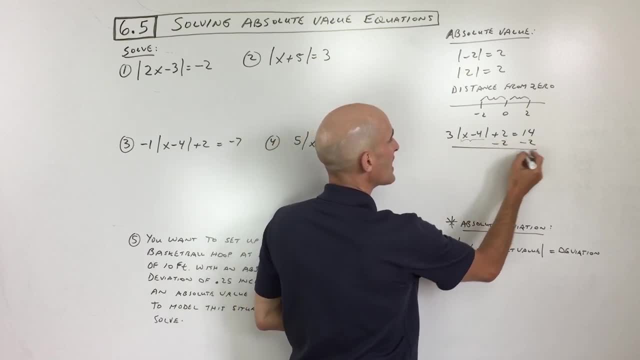 is, I'm going to work from the outside in, I'm going to subtract two from both sides. That way those cancel. so that gives us 12. And here I'm going to divide both sides by three, okay, because we're trying to get that absolute value quantity. 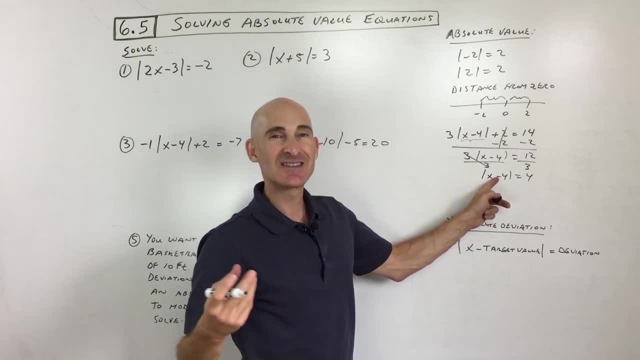 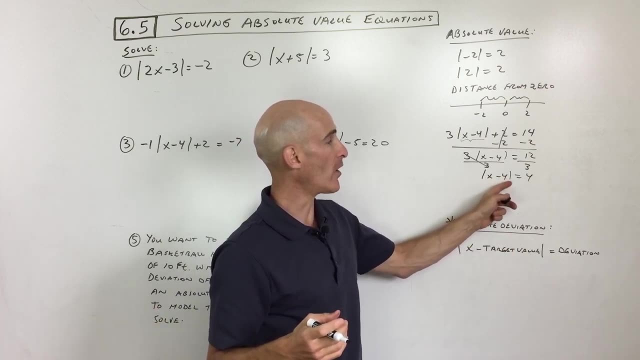 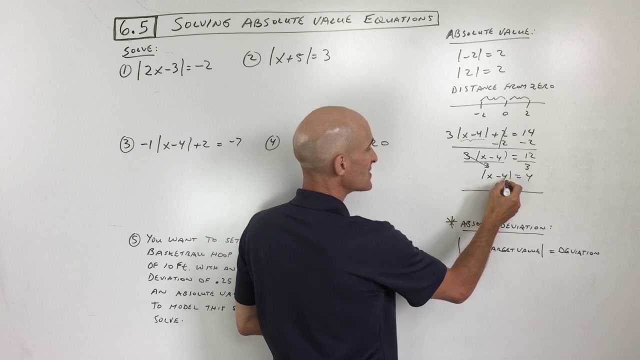 Now what this represents here. see, minus means the difference, and difference means the distance. okay, in geometry, So the distance between some number and four is four units. So if you think about this, on the number line, here's four and the distance between some. 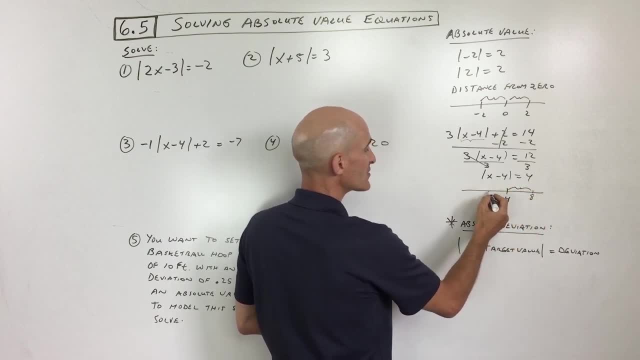 number and four is four units. So it means it could be four units to the right, It could be four units to the left. So you can see that the answer is going to be either zero or it's going to be eight, And you can double check that. See zero minus. 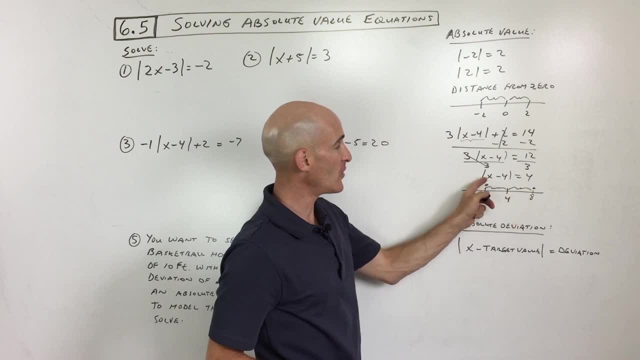 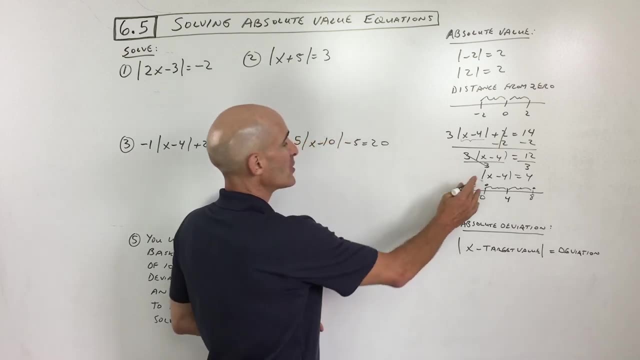 four is negative four, but when we take the absolute value, it makes it positive four. If we do eight minus four, that's four. The absolute value of four is still four. It always gives us a positive result. Now, if I was going to solve this, I wouldn't do it geometrically. 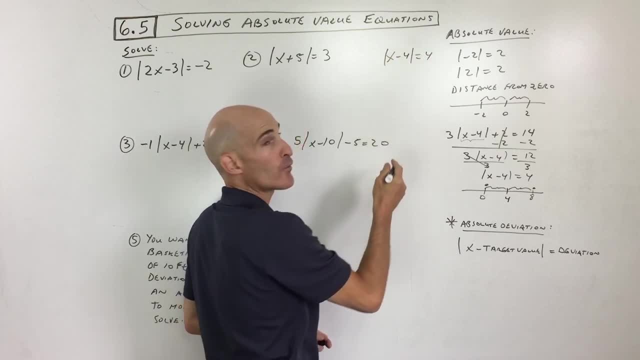 like that. I would just do the algebra method. I would say: x minus four equals four. What you want to do is you want to split this up into two equations: x minus four is equal to positive four or x minus four is equal to negative four. Then you just add four to 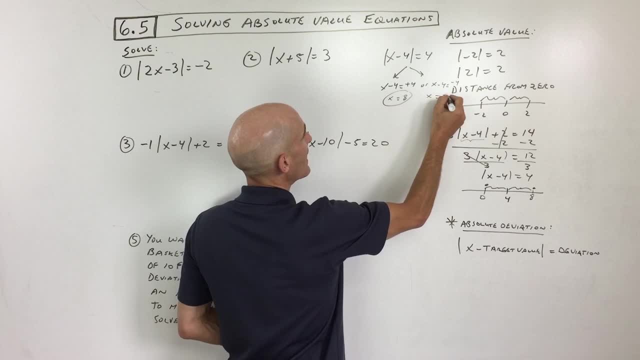 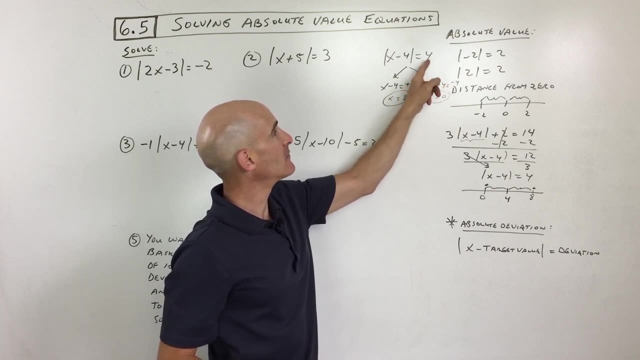 both sides, We get x equals eight. Add four to both sides, We get x equals zero. So that's the key is, you want to split it up into two equations, one with the positive scenario, one with the negative scenario. Because, remember, whatever 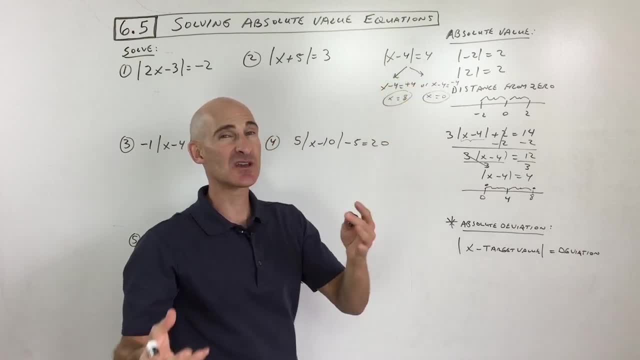 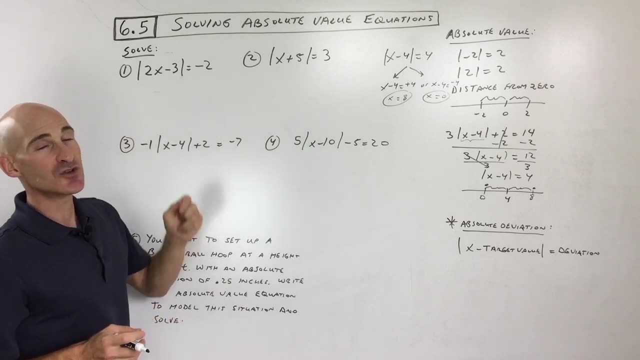 was in here originally. if it was negative, when we take the absolute value it's going to make it positive. So we consider both cases. I'll show you some examples. Say, for example, this one: here, the absolute value of two x minus three is equal to negative two. Well, 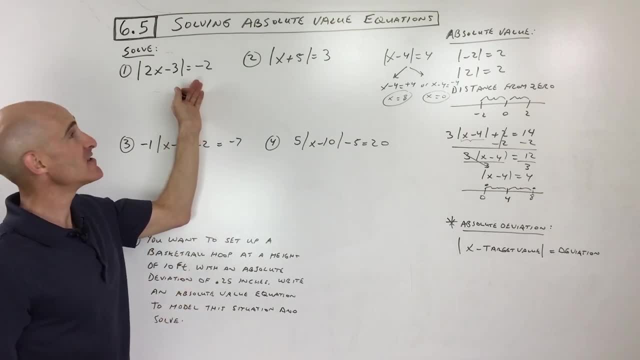 this one's actually a trick question And I put this in here on purpose because sometimes you'll see this: When we take the absolute value, remember how we talked about how it always has to be positive. You can never have a negative value when you take the absolute value. So this one is actually 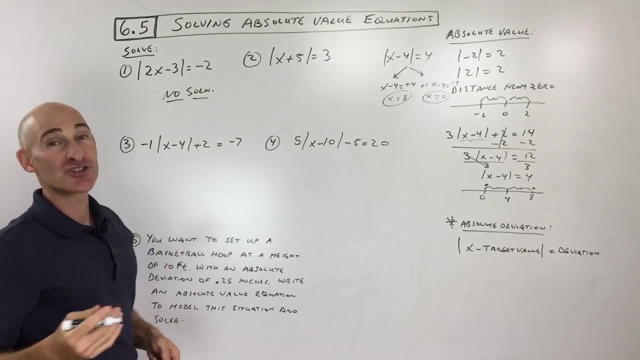 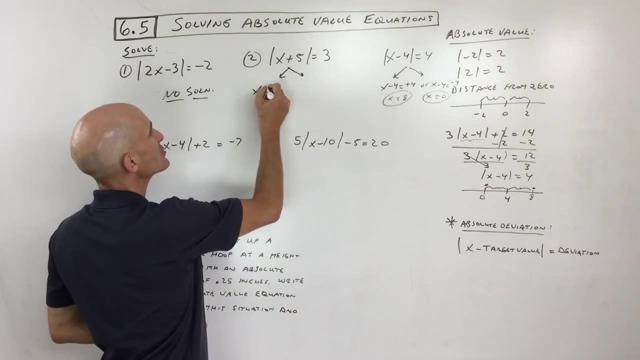 no solution, And I wanted to show you that in case you ever see something like that. So now number two. let's do this one. So this one. what we're going to do is we're going to split it up into two equations: x plus five equals three, or x plus five equals negative. 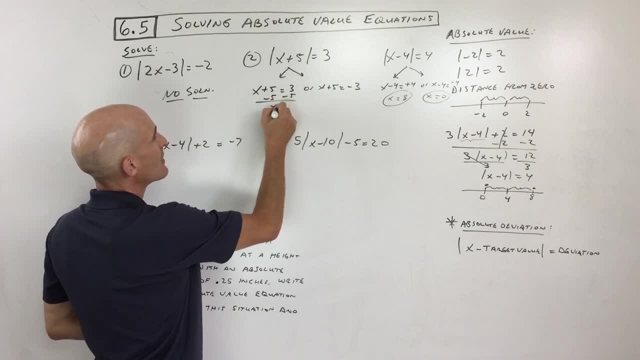 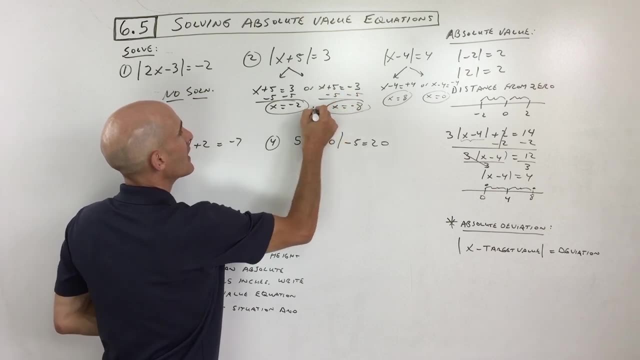 three. All we have to do is solve these equations separately. So that's x equals negative two or subtract five from both sides. here We get x equals negative eight, And I'm just going to put the or in between. So x equals negative two or x equals negative eight. Now the nice thing about algebra is you can check. 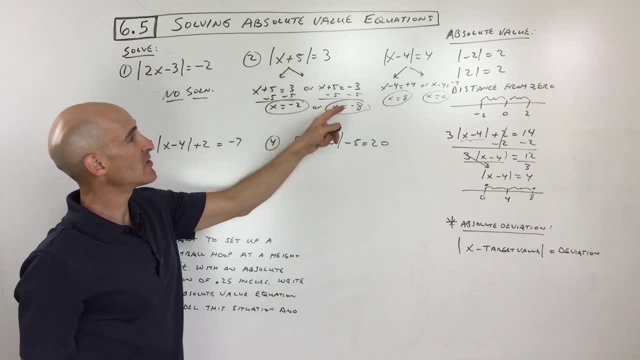 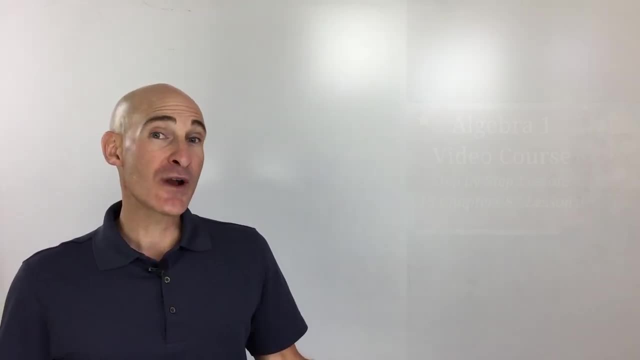 your answer. You put it back in Negative: two plus five is three. Absolute value of three is three. Negative eight plus five is negative three. Absolute value of negative three still gives us positive three. But the key is to split. Want to learn algebra one? 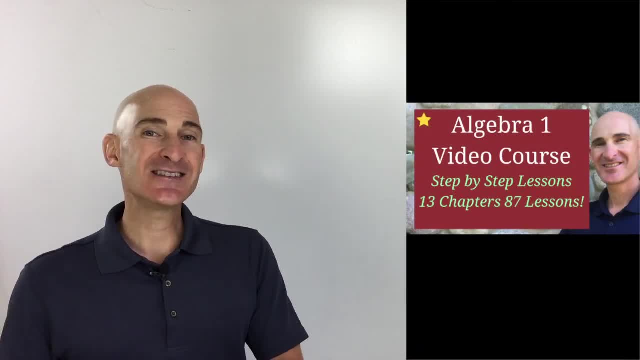 Check out my learn algebra one video course for sale, where we go through 87 video lessons that take you step by step by step through algebra one. We talk about the important concepts, formulas and we go through numerous example problems together to help you learn algebra. 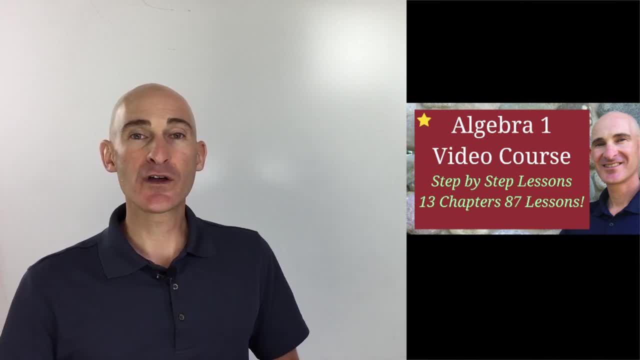 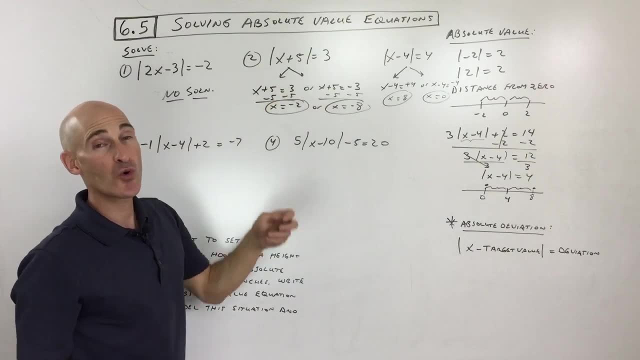 one Click the interactive card or the link in the description below to take you over there to get started with some of the free lessons. In the meantime, let's continue on with this video, But the key is to split it up into two equations and consider the positive. 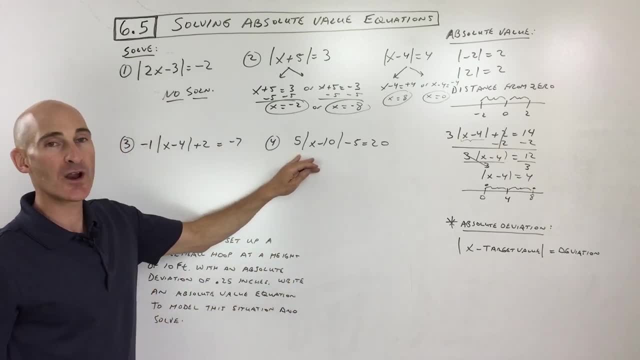 case and the negative case. See if you can do number three and number four on your own, We'll go through them here together. So again, our goal is to get that part in absolute value by itself. So I'm going to work from the outside in by doing the opposite operation. So I'm 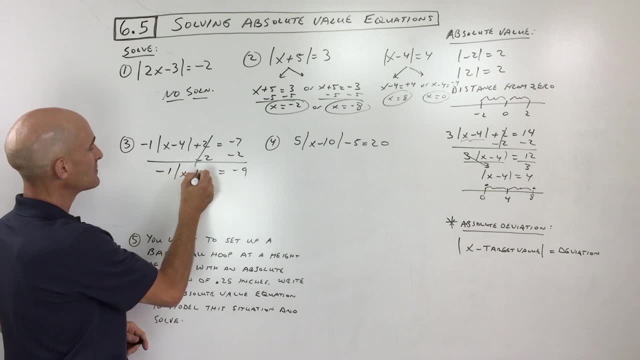 subtracting two from both sides. Now I'm going to multiply both sides by negative one, So that's going to give you x minus four equals positive nine. Now I'm going to split it up into two equations: x minus four equals nine, or x minus four equals the opposite of nine. 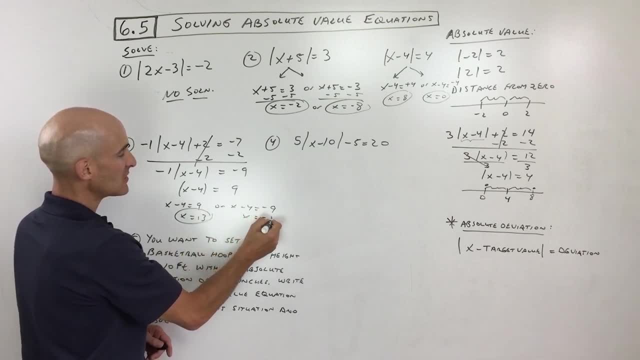 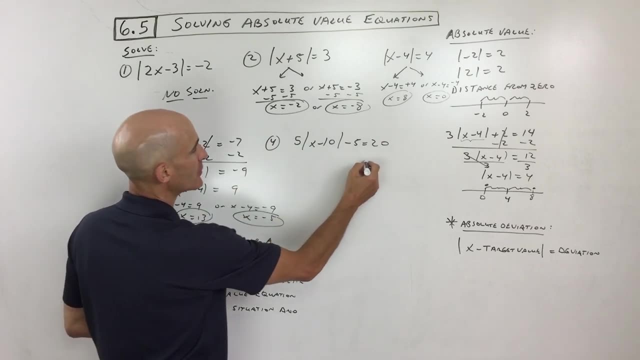 Add four to both sides, we get 13.. Add four to both sides, we get negative five. And those are our two solutions. And again you can plug them back in and check. Let's look at number four, See if you can do this one on your own. 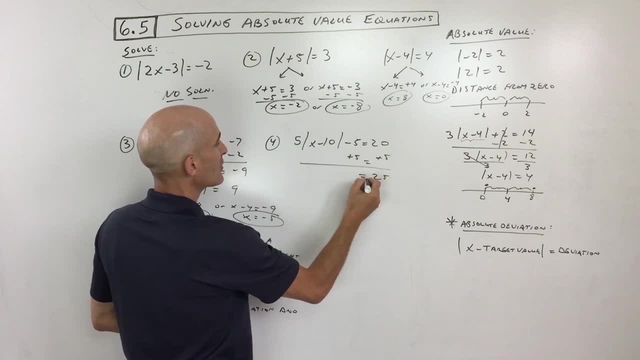 Again, working from the outside, in trying to get that absolute value portion by itself. looking at one side of the equation, I'm going to do the opposite of multiplying by five, I'm going to divide by five. So 25 divided by five is five X minus 10.. Now we split it up into two equations. 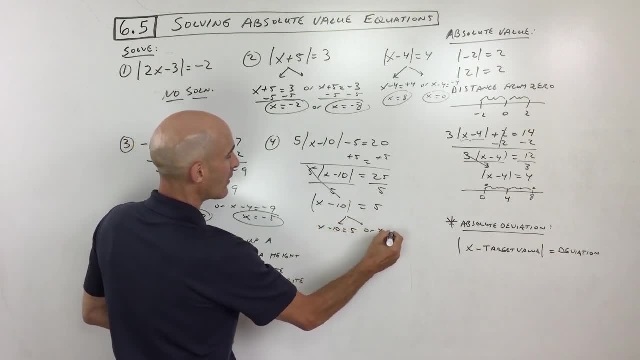 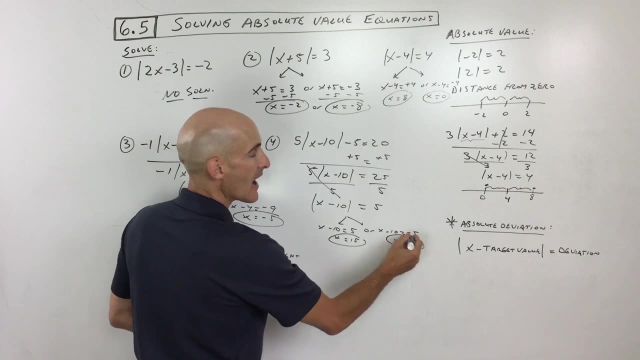 right. X minus 10 equals five, or x minus 10 equals negative five. Add 10 to both sides, we get 15.. Add 10 to both sides, we get five, And you've got it. So one last problem here. 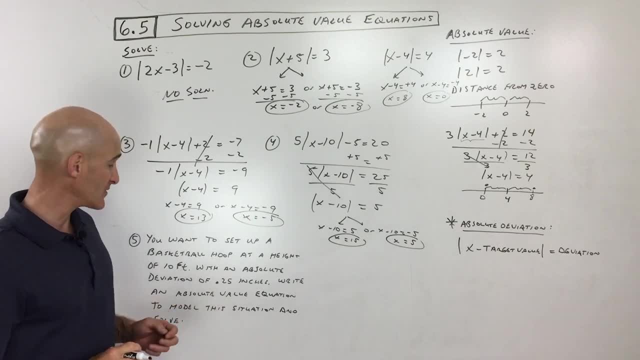 in this section we're going to do a word problem. Of course we've got to get good at our story problems. You want to set up a basketball hoop at a height of 10 feet with an absolute deviation of 0.25 inches? okay, Write an absolute value equation to model the situation. 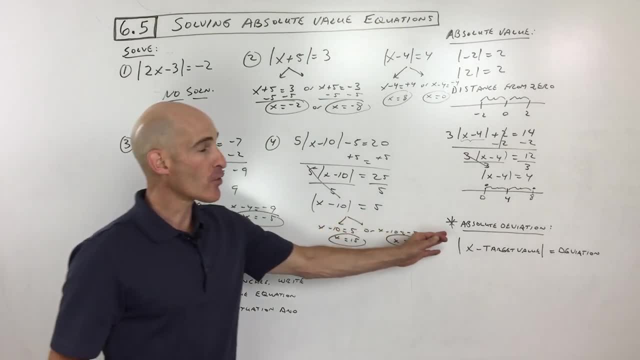 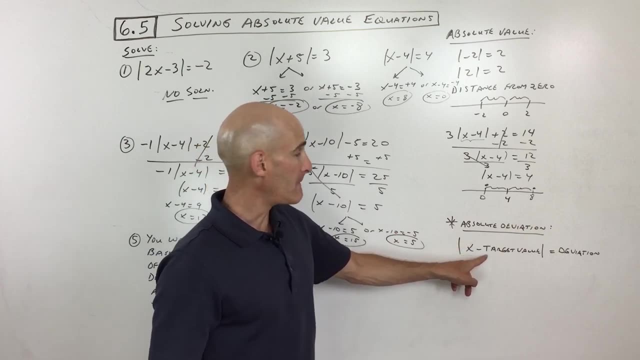 and solve. Okay. so let me just show you a formula that's going to be really helpful for you. It's this one right here, this absolute deviation equation X is your variable minus your target value. That's what you're aiming for. That's going to give you whatever the value of your target. 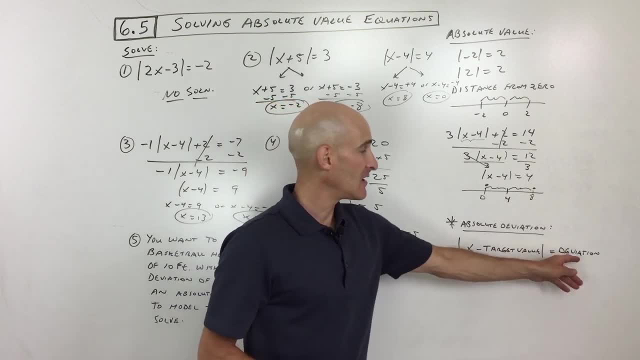 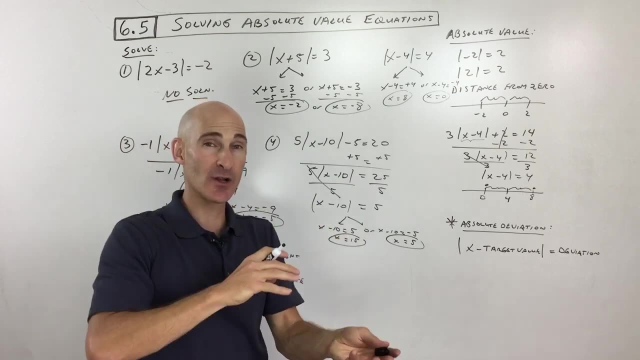 So you're going to get an x minus six. Now it's going to be x minus six. So what you're that difference? okay is the deviation. So deviation means how far off are you? Like you could be a little bit higher, the basketball hoop could be a little bit higher, or it could be a 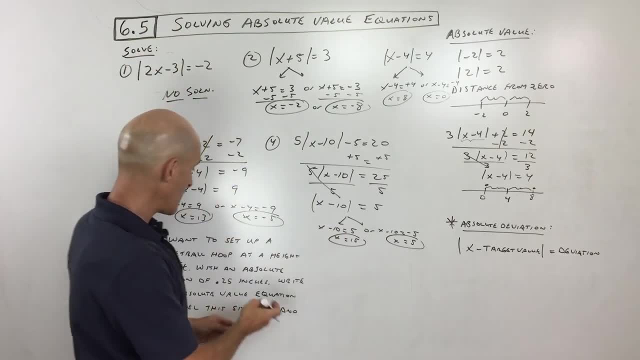 little bit lower, but you don't want it to be higher by more than 0.25 inches. You don't want it to be lower, you know, by more than 0.25 inches. So if we're going to write this, we're. 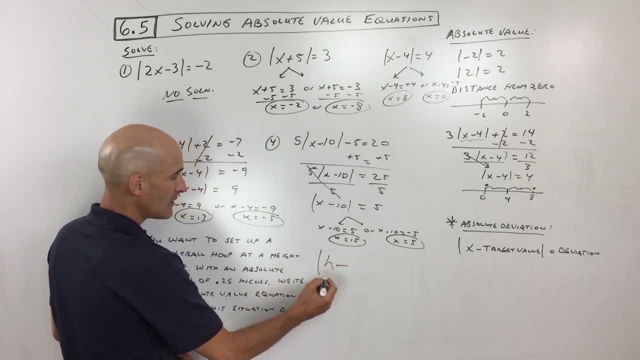 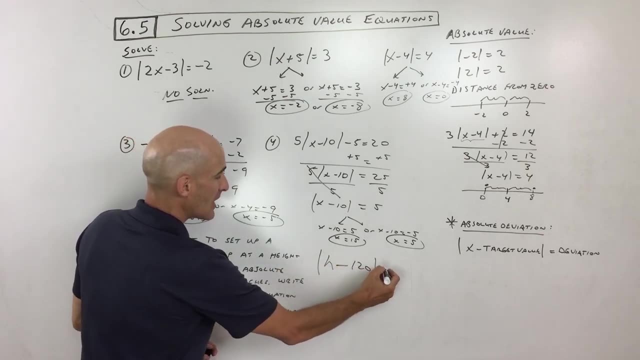 going to say I'll just use H for height. So the actual height minus our target height, which is 10 feet- I'm going to convert that to inches, that's 120 inches is equal to the deviation We don't want. we want it to be. we want it not to be off by more than 0.25, but in this case, 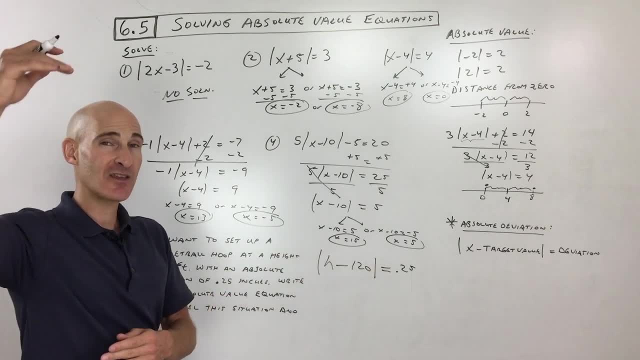 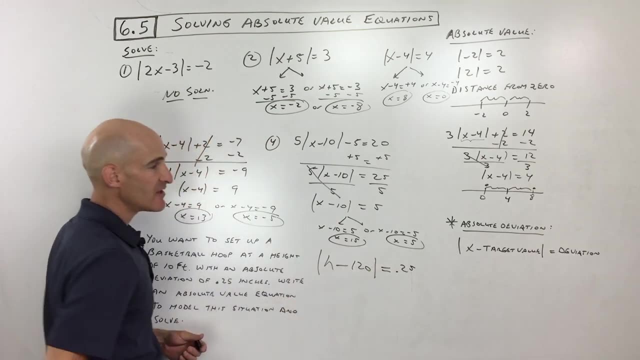 we're just going to set it equal to 0.25 to figure out what the maximum height the hoop could be at, and then the minimum height. Okay, so that's it. So it's our variable minus our target value equals our deviation. Now, the reason I converted this to inches is because this was in inches.